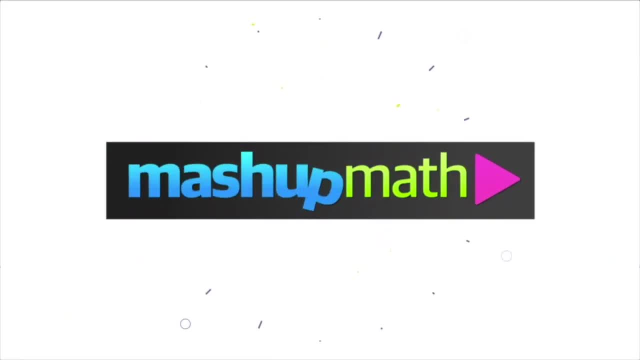 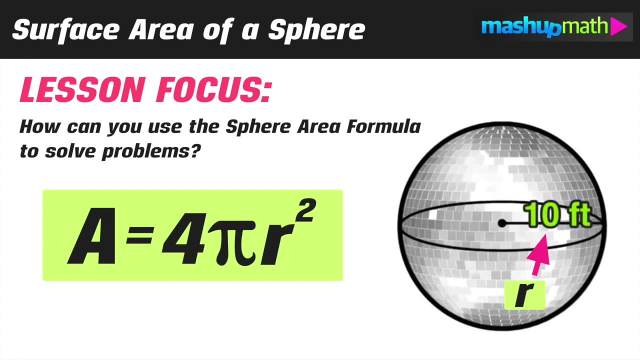 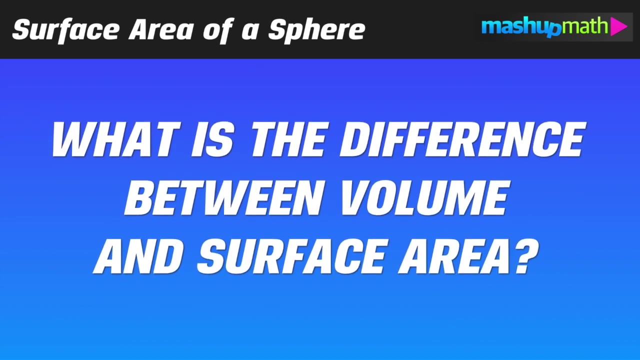 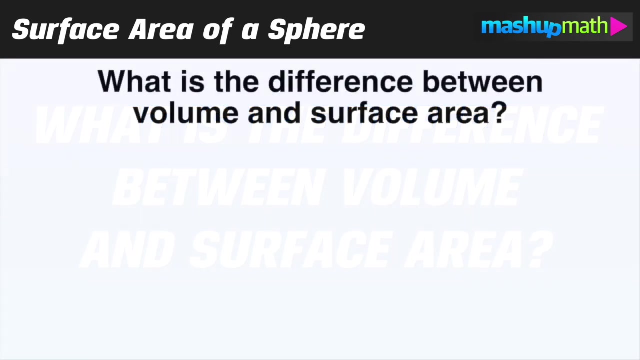 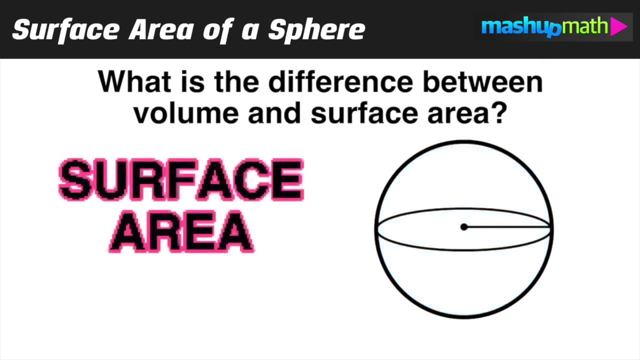 Let's go ahead and ask the question: what is the difference between volume and surface area? Now, the volume of a sphere refers to how much room is inside of it. Imagine that we wanted to fill it up with water completely. Now, surface area refers to the outside, as if we wanted to know how much space to cover. 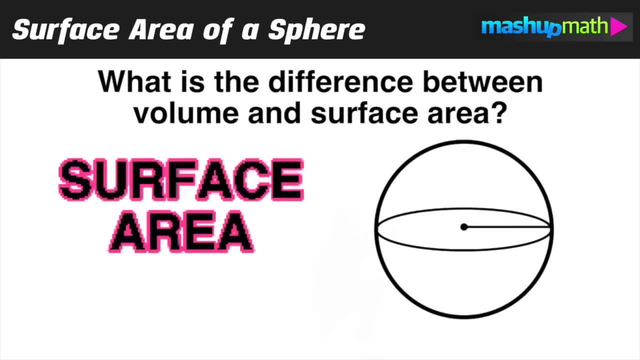 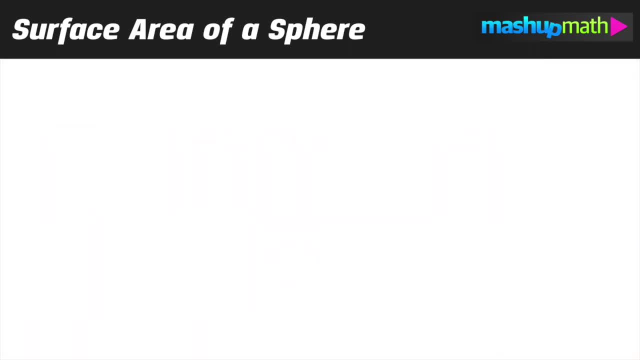 the entire outside of the sphere, like if we wanted to spray paint the entire thing orange. Now there are two formulas that we are going to have to reference to find volume and surface area of a sphere. The formula for finding volume of a sphere is 4 over 3 pi r cubed. 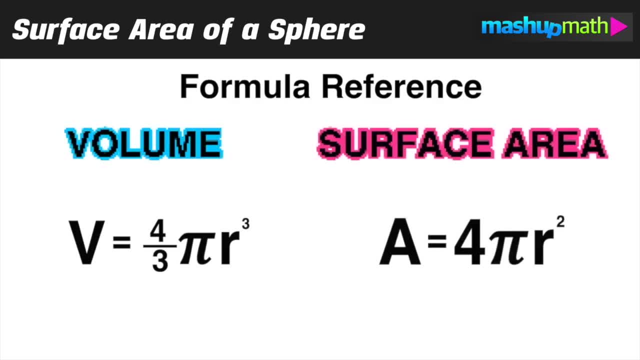 and the formula for surface area is 4, pi r squared. Now notice the exponents for each formula. Volume is cubed, surface area is squared, So when we express an answer, we have to use appropriate units. So volume is going to be in cubic units and surface area is going to be expressed in square units. and 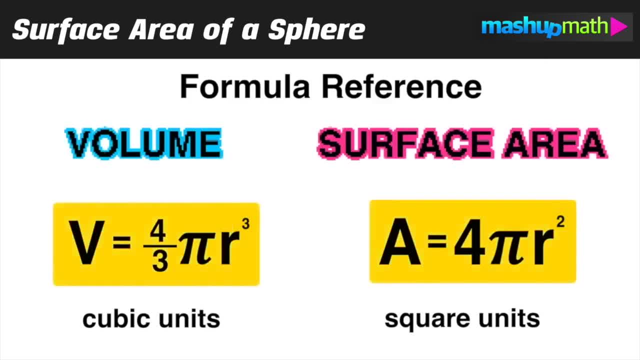 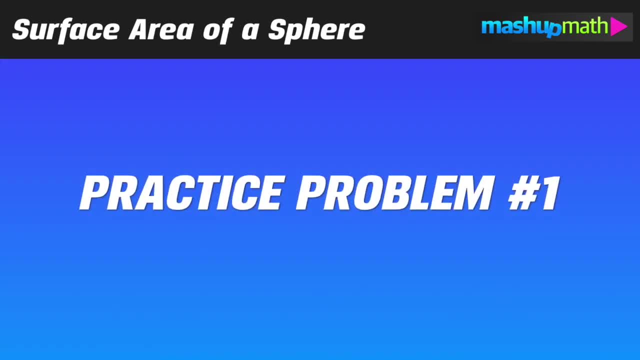 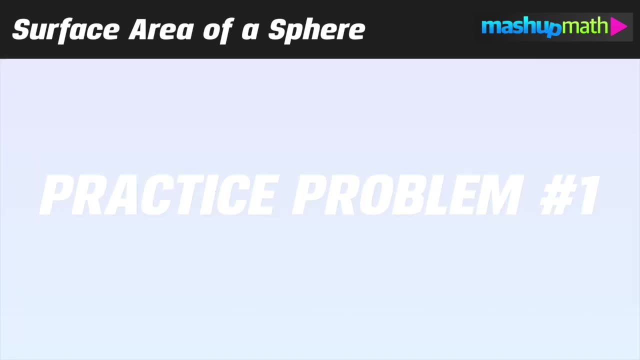 again, that correlates with the exponent in the formula. So make sure you have these two formulas available, because we are going to apply them now in these next two examples. So in our first example we want to find what is the surface area of a disco ball with a. 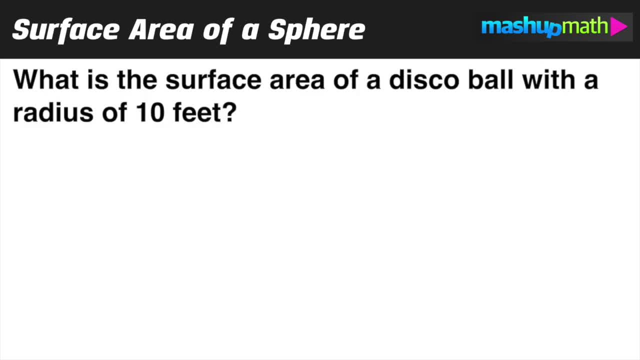 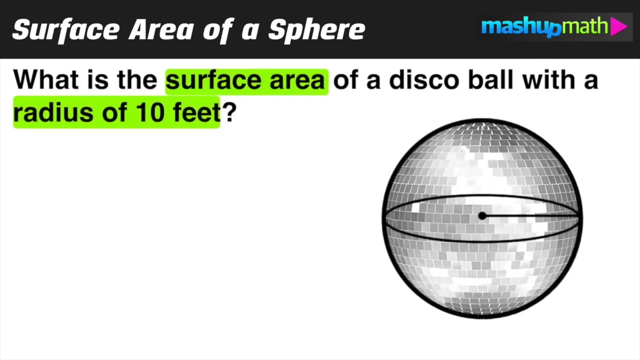 radius of 1. Of 10 feet. So it's always a good idea to start off by identifying the key information. In this case, we want to find surface area and our radius is going to be 10.. Now we know that a disco ball is a sphere, so we need a diagram. So we will go ahead. 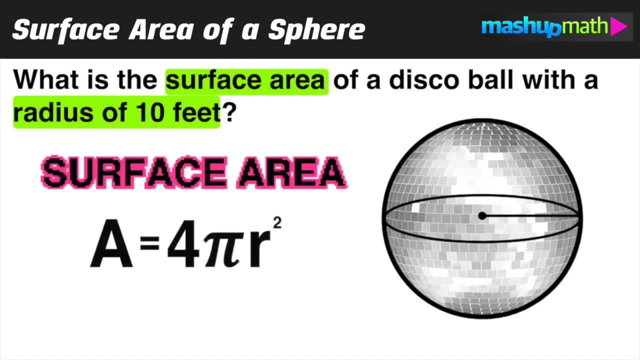 and set that up, and we know that we want to find surface area, so we are going to be using the surface area formula of a equals 4 pi r squared. Now we know that the radius is equal to 10 feet, so we can go ahead and label that on.